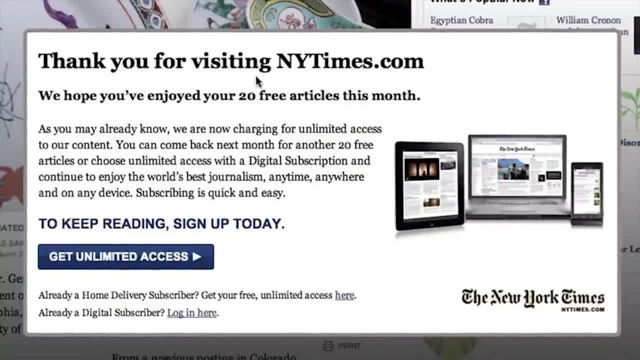 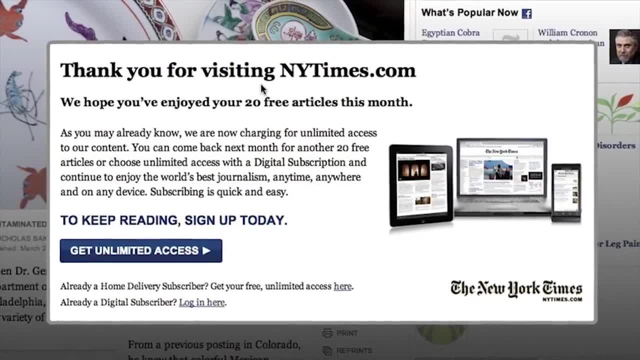 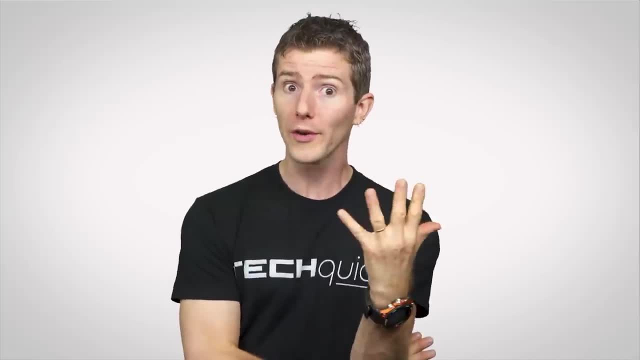 advertisers from snooping on what you're looking at and even get around website paywalls on sites that use cookies to track how many articles you've viewed before they start charging you. Newspaper websites are notorious for this last one. However, you've probably seen the warnings that pop up in incognito mode telling you. 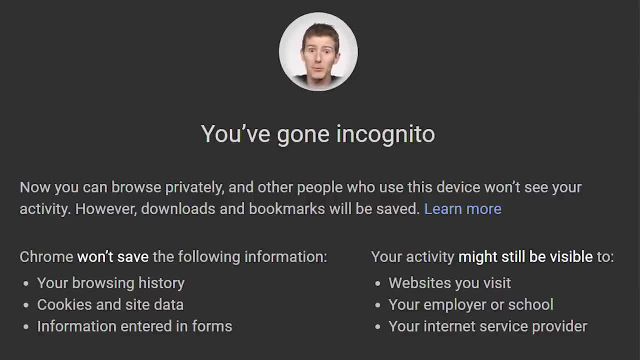 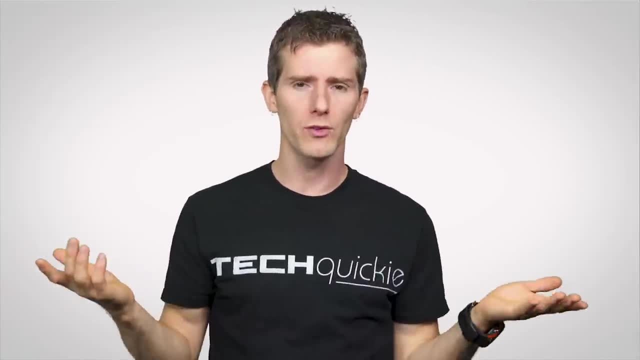 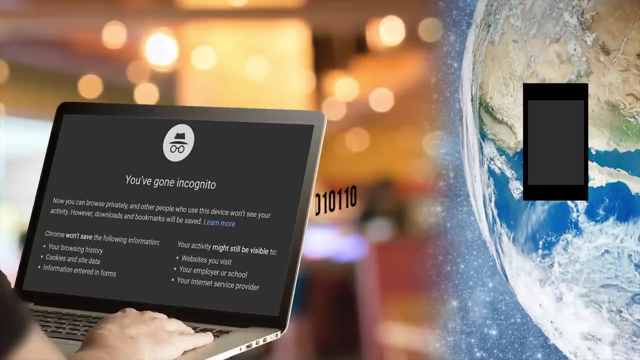 your employer or internet service provider might still be able to keep tabs on your online activity. Well, how would they do that? Well, because incognito mode only affects what's being stored locally on your computer. all of that traffic is still being routed through the servers at your ISP and 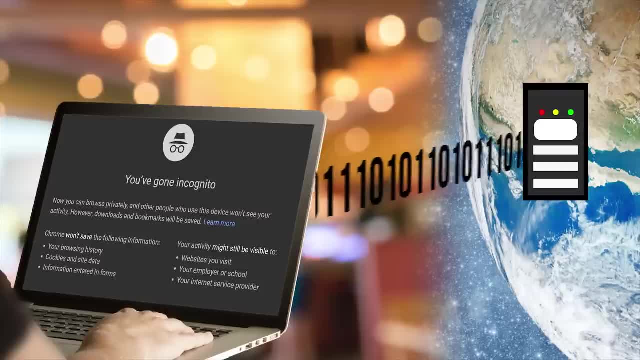 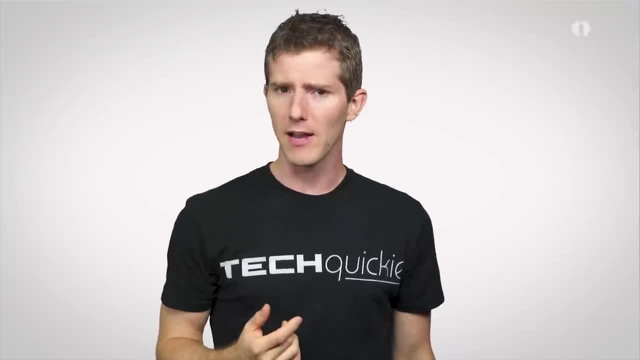 also perhaps your school or office, so it can still be intercepted and tracked. You can learn more about that right up here. So that means that if you really want to anonymize your web traffic, you'll need to consider using a VPN as well. 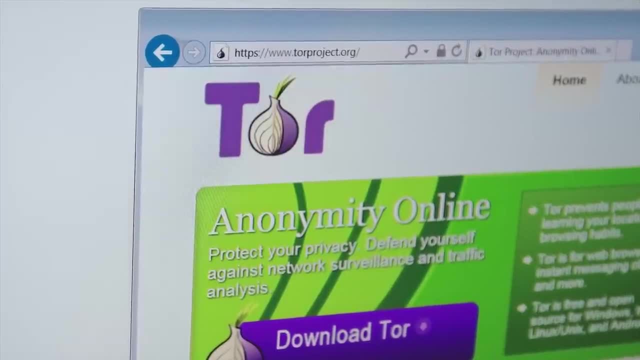 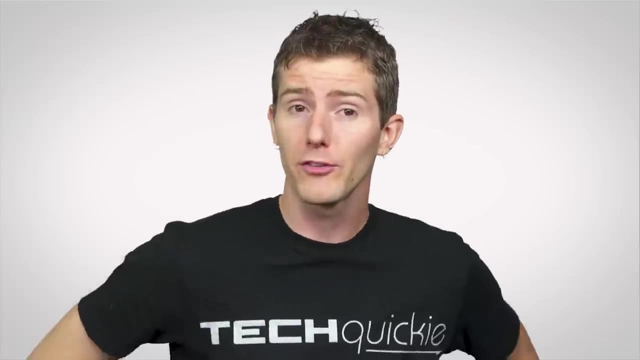 possibly over a network like Tor to further conceal your identity. Also, remember that just because a browser deletes the information about your session doesn't mean it will keep a determined snoop from finding out what you've been up to, For example. 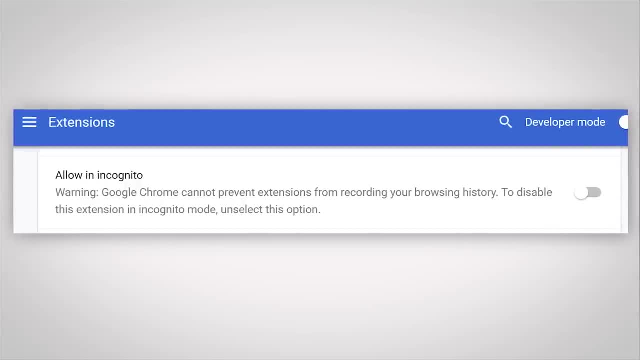 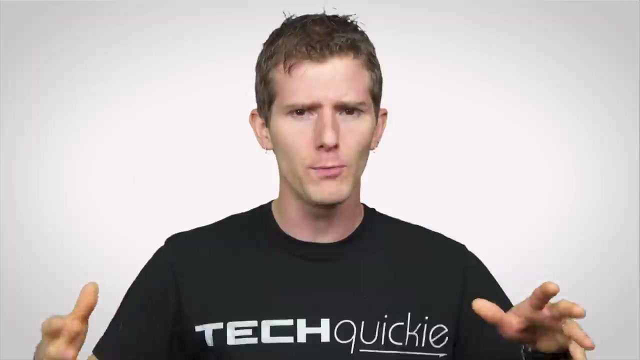 features that can run in incognito mode, such as browser extensions or Adobe Flash, can still leave visible traces on your computer unless you make sure that those are disabled as well, And browsers also don't necessarily delete any data that you built up during an incognito session securely. 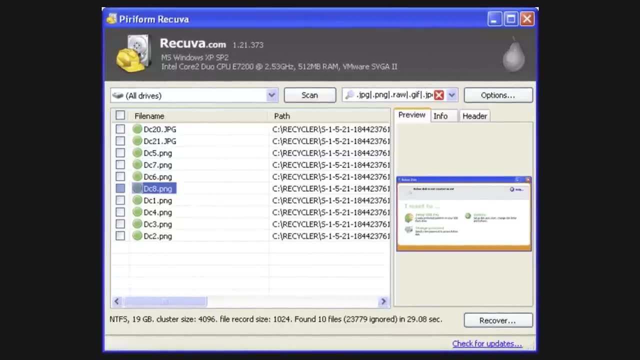 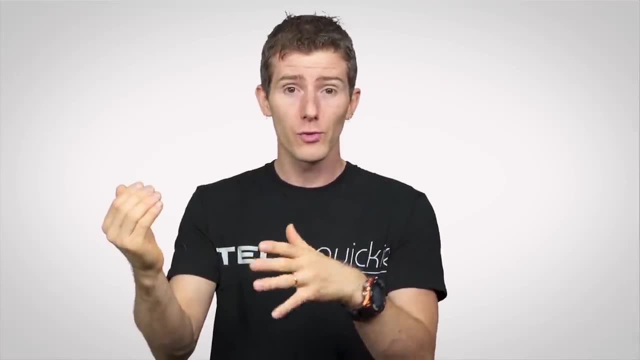 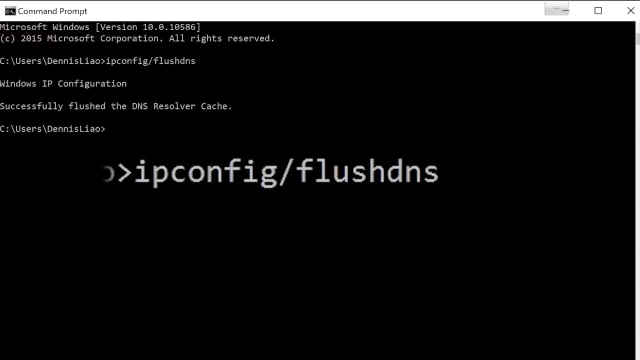 So some of it could still be found with a software recovery program or inside your PC's DNS cache, which matches the URLs of the sites you visit to the IP addresses. So you'll need to make sure that you clear your DNS cache with this command if you're really worried about privacy. 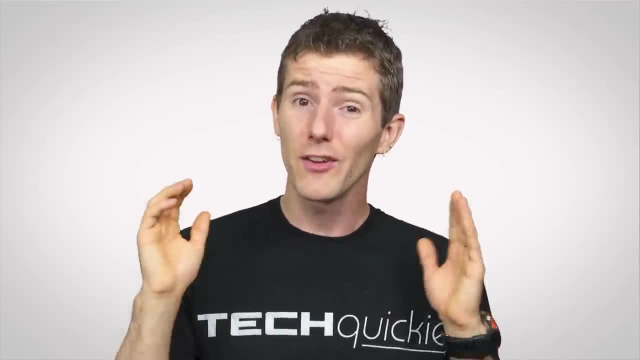 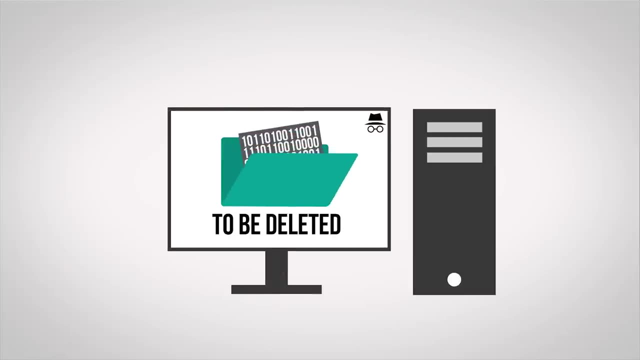 Finally, things that go wrong on your PC can also compromise the effectiveness of incognito mode, Since many browsers delete the data from your incognito mode session once you close your session. an unexpected error, like a computer crash, could keep that data from being deleted normally. And then, of course, any malware or 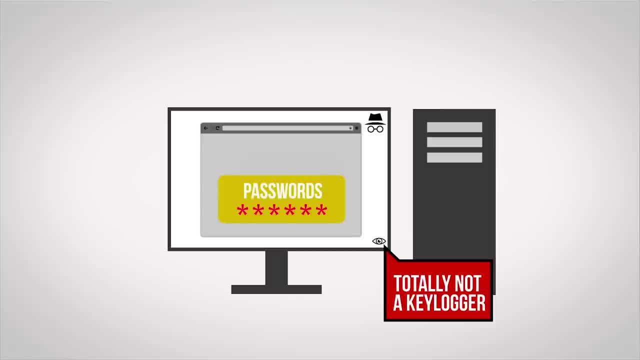 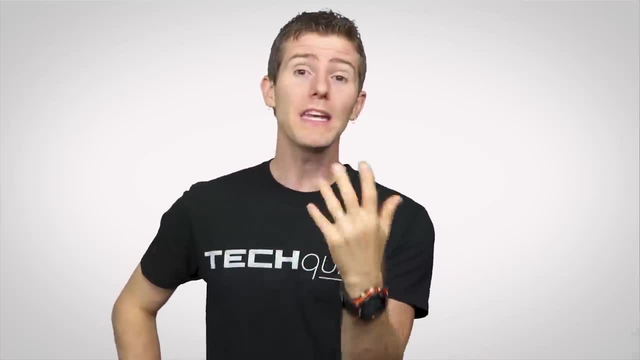 spying software like a key logger could easily be keeping tabs on your incognito browsing if your PC is infected. Now we're not trying to scare you or make you think that private browsing is useless. It's still a powerful tool and an easy, quick layer of security.